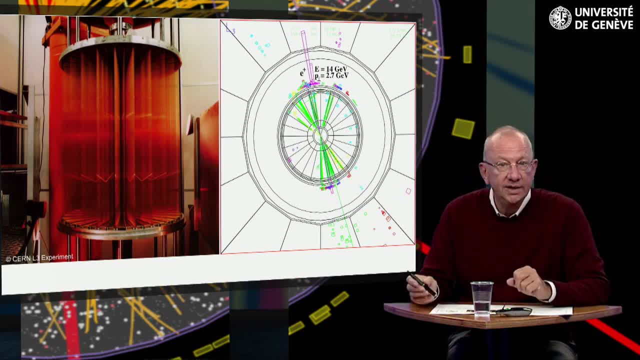 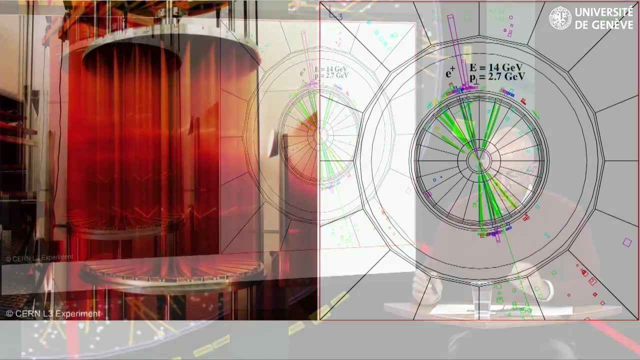 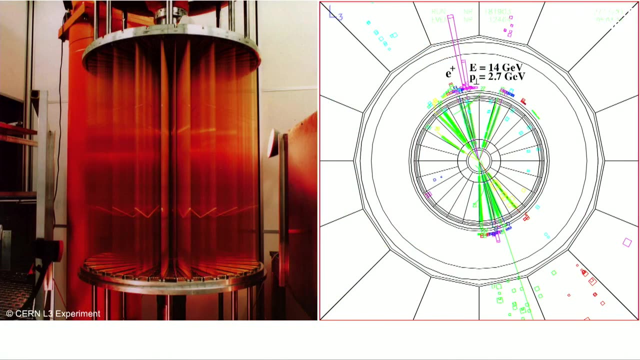 The reaction takes place in the middle of the device, the center of the image. on the right, In the central part, you see the tracks of charged particles in yellow, reconstructed from the measured coordinates indicated by the small green crosses. The curvature is barely visible but well measured by the high-resolution drift chamber. 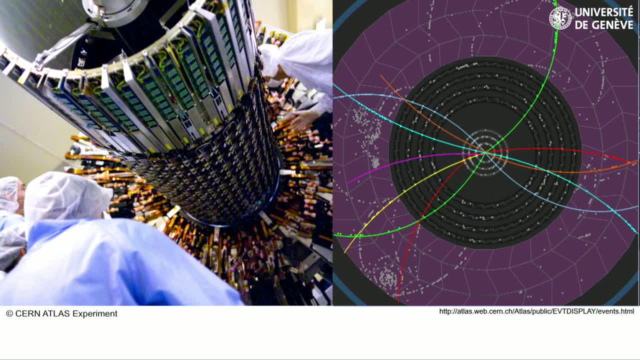 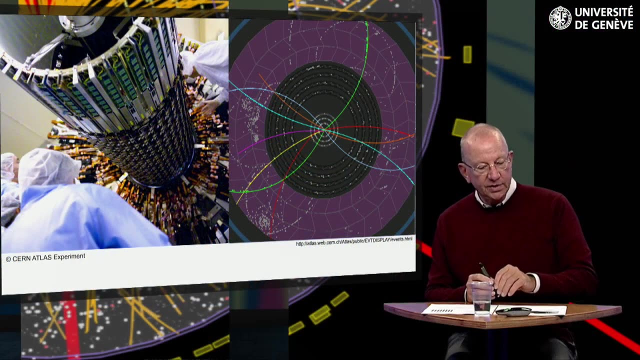 In the graph on the left you see a central detector made out of silicon sensors, the one that is used by the ATLAS experiment. The right image is the reconstruction of a reaction between protons in the middle of the device. The charged particles which are produced leave tracks forming circles orthogonal to 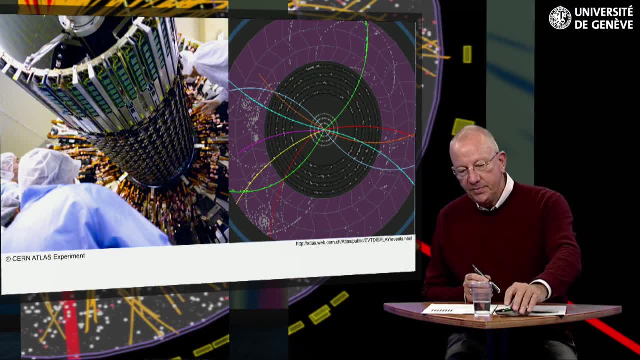 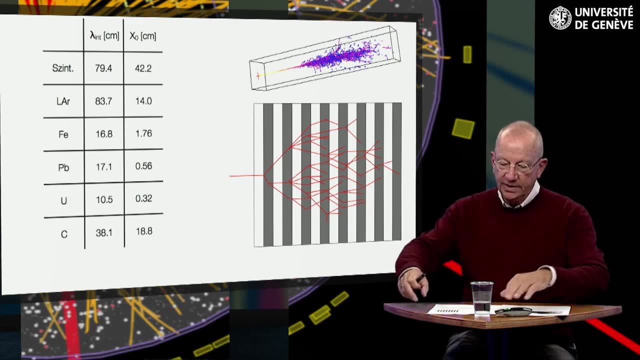 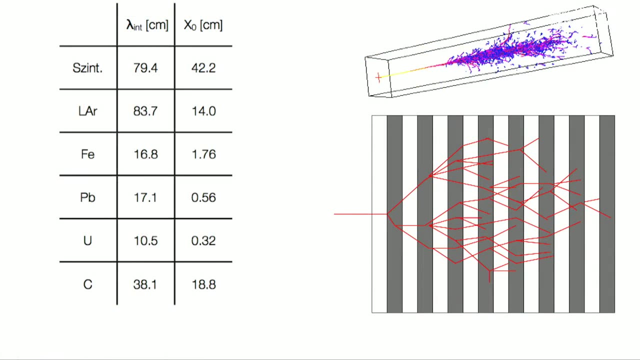 the magnetic field. The purpose of a colorimeter is to measure the energy and direction of particles by absorbing them. The principle of operation is the following: The incident particle initiates a shower of particles in the detector- an electromagnetic shower or a hydronic shower. 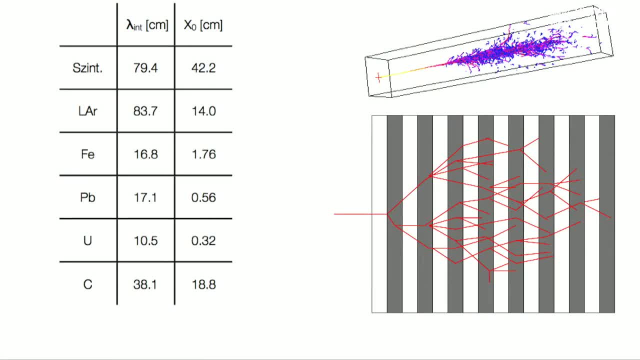 The shape, size and composition of the shower depends on the incident particle, but also on the detector materials, namely its radiation length, its nuclear interaction length. The energy is deposited in the form of heat, which is not very useful but also produces 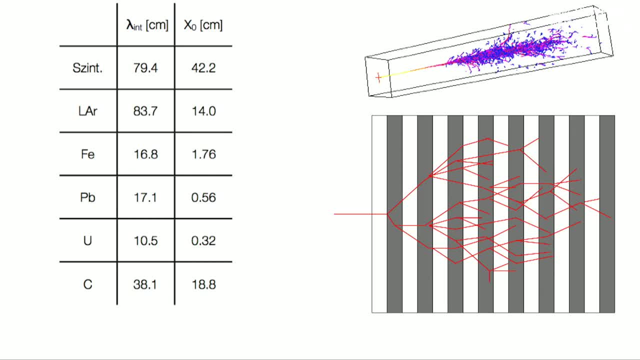 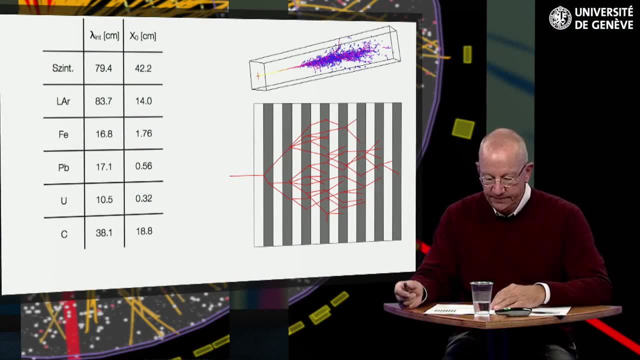 detectable signals. These signals, like ionization and excitation by the EDX, scintillation light, Cherenkov radiation, etc. This energy is detected by sensors. The resulting signal is proportional to the total energy deposited by the particle of. 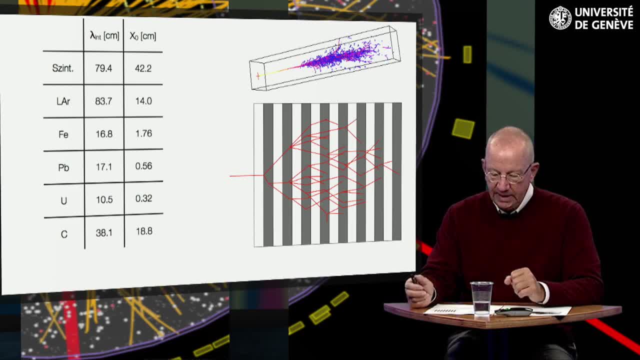 the shower in the active medium of the detector. There are two kinds of colorimeters: homogeneous ones, with only one material to absorb and detect the shower particles, and layered colorimeters, which use different materials for interaction or absorption. Here is an example of a layered colorimeter. 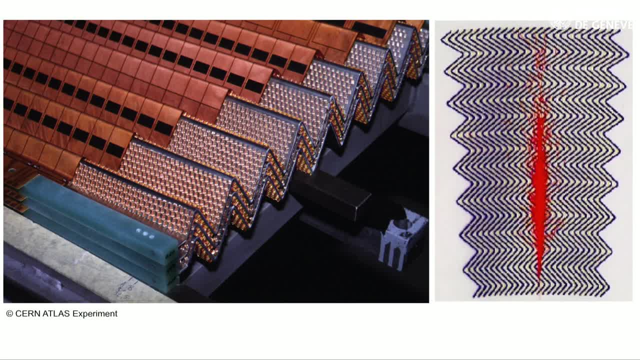 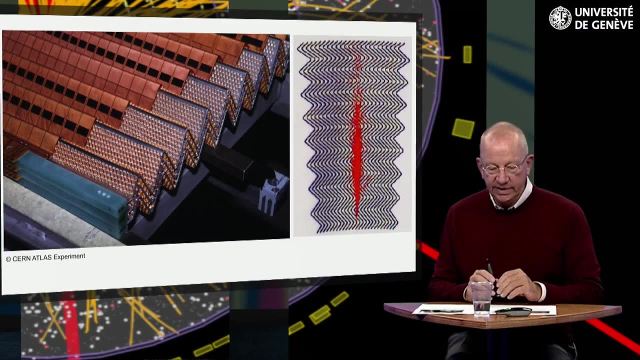 In such a colorimeter, layers alternate. There are absorption layers made of heavy materials like copper, lead or uranium with a short radiation and hadron interaction length. Here particles interact and form the shower. In the sensitive layers the energy lost by the EDX is recorded. 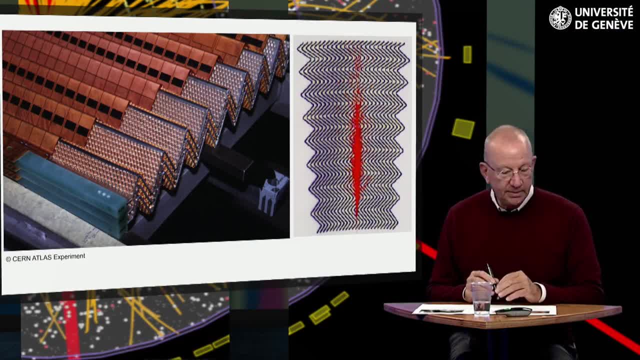 These layers may be equipped with a gaseous or noble liquid particle. The energy is also recorded. There is a proportional chamber, a semiconductor sensor or a scintillator. You see here the electromagnetic colorimeter of ATLAS, which contains absorption layers. 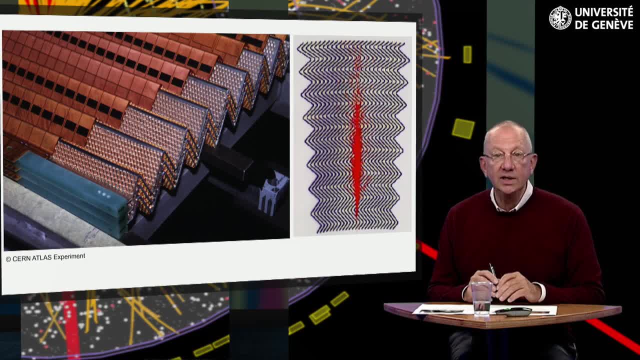 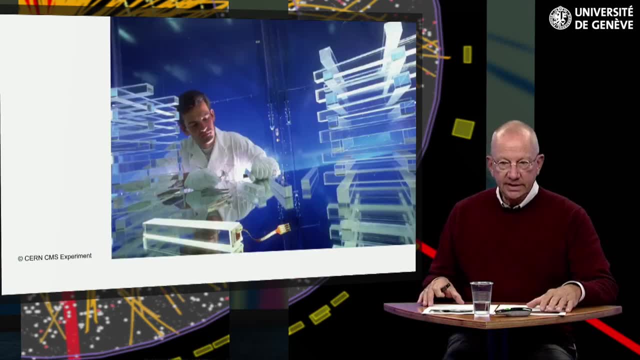 of lead and steel, alternating with sensitive layers filled with liquid argon. The whole has a shape resembling an accordion In a homogeneous colorimeter. on the other hand, the two functions are combined: The same material is used as an absorber and as a detector for deposited energy. 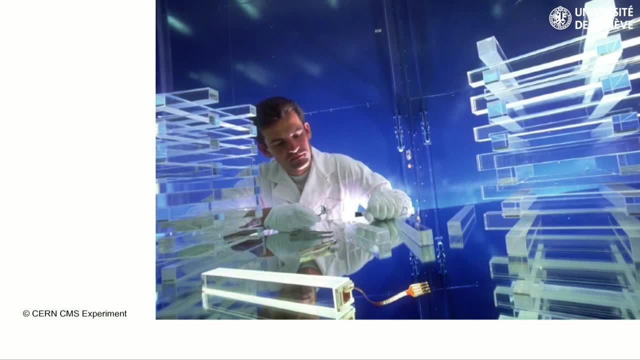 Scintillators made of heavy materials can be used to detect the shower particles. These materials can be used like bismuth-germanate or lead-tungstate. Because of the short radiation length and the transparency of these materials, they are often used to detect electromagnetic showers. 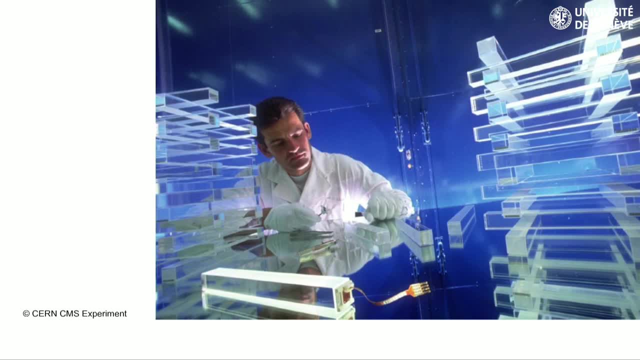 The scintillation light emitted by the electrons of the shower is detected either by photomultipliers or by semiconductor photodiodes, as in this example, which shows you the lead-tungstate colorimeter of the CMS experiment at the LHC. 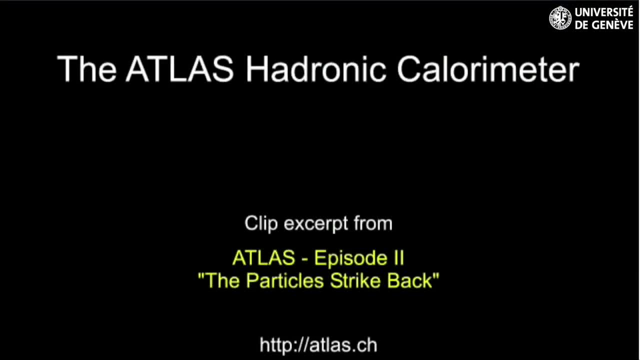 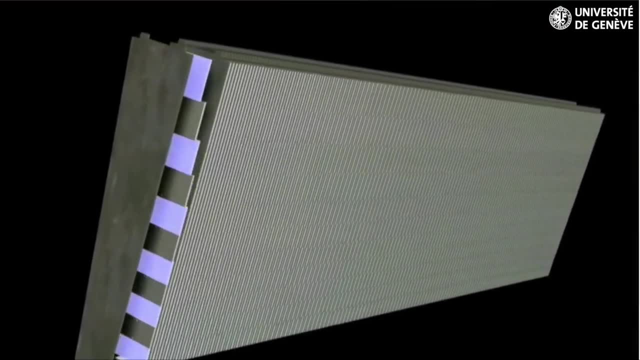 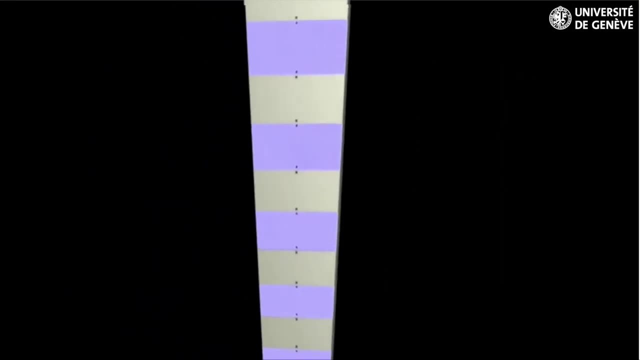 Colorimeters are also one of the main applications of plastic scintillators. The Large Colorimeter for Hadron Showers of the ATLAS experiment is an example. Here you see a small animation showing the structure of one of its wedge-shaped slices. 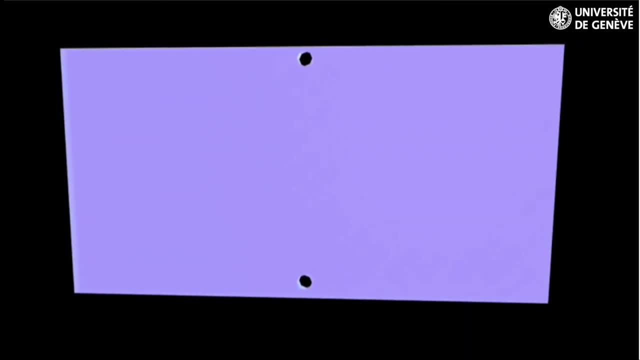 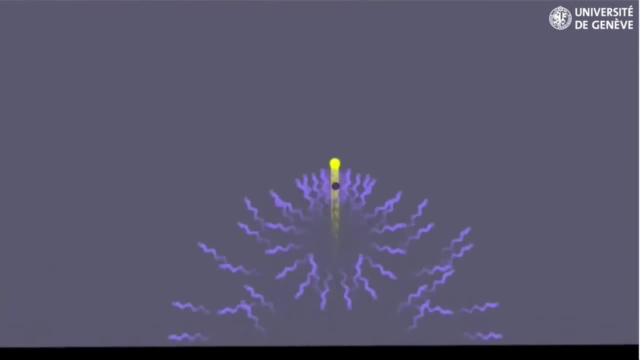 It uses scintillator tiles inserted between steel absorbers to measure the energy of hadrons. The shower develops mainly in the metal layers. The charged particles it generates are the energy of the hadrons. The shower develops mainly in the metal layers. The charge- обратic approve-activatorранsuwates produce scintillation light in the sensitive. 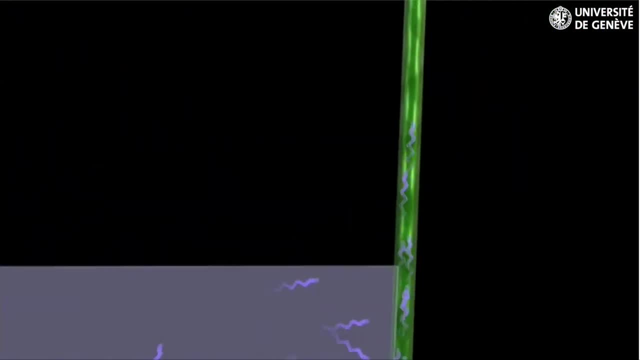 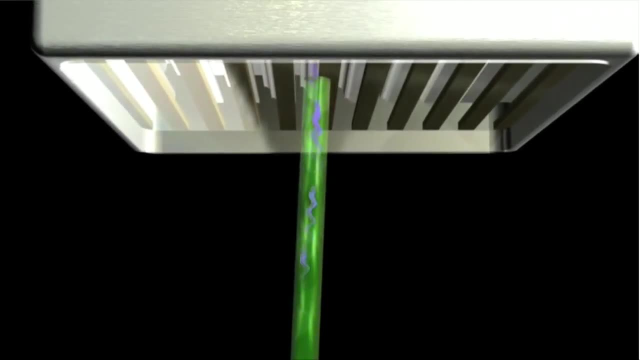 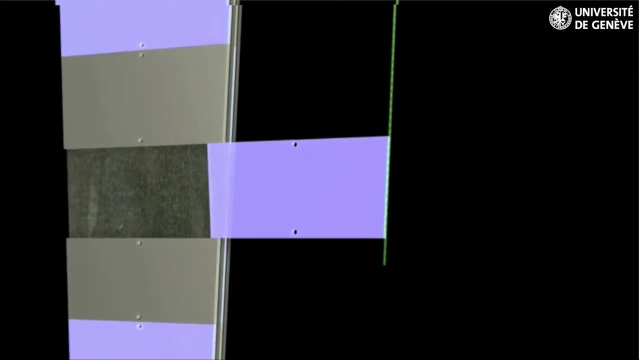 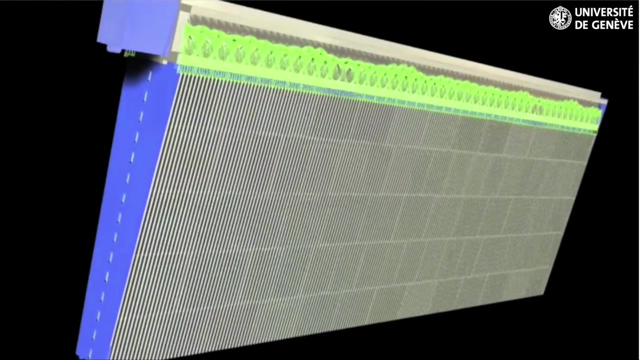 layers. The scintillation light is collected by optical fibers and guided to the photodetector, in which a three-dimensional image of the shower is measured, which allows to reconstruct the direction- and energy of hadrons. But also the Cherenkov effect allows to build complete detectors. 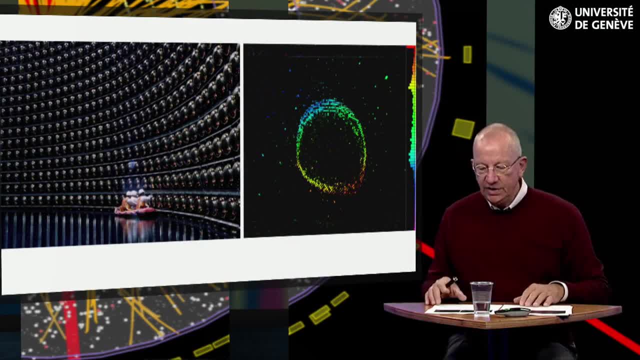 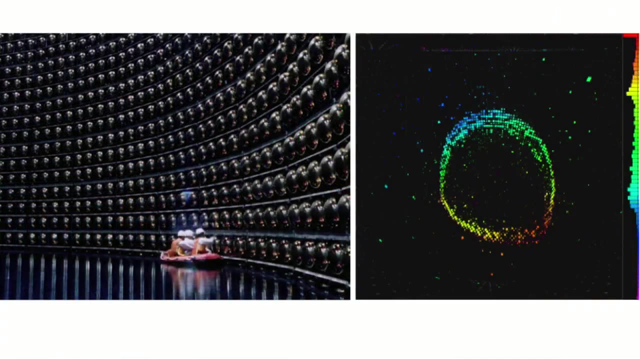 The Super-Kamiokande detector in Japan consists of a huge cylindrical tank which contains 50,000 tons of ultra-pure water. When a charged particle passes through the water at a speed beyond that of the speed of light in water, which is about 75% of the speed of light in vacuum, a cone of Cherenkov light is emitted.